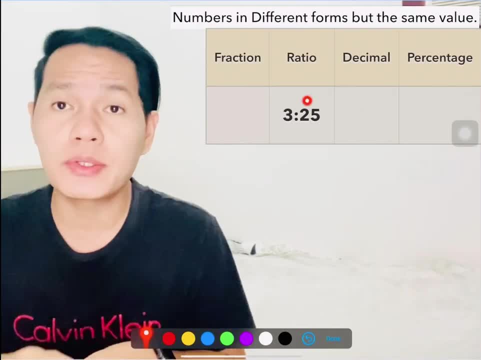 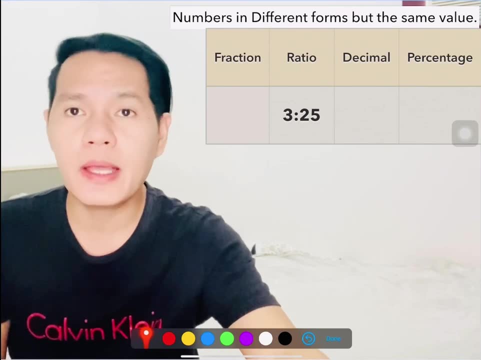 next one, Next up, guys, is how are we going to change this ratio 3 to 25 into fraction, into decimal and into percentage? Okay now, first thing is very simple: Just change this first into fraction, because this is already in ratio, So just simply write it into 3 over 25.. 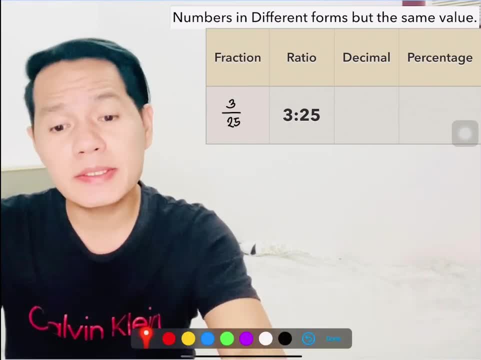 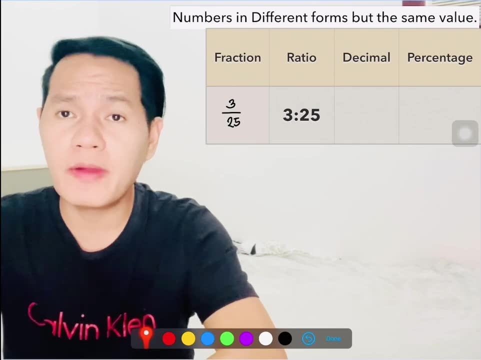 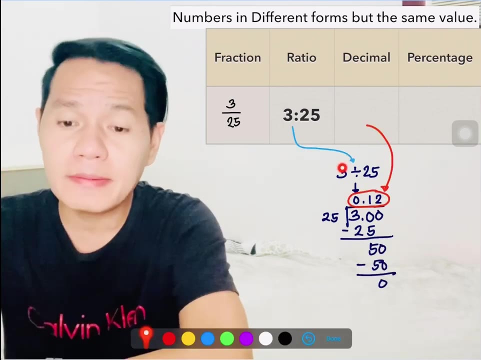 That's it, The next- into decimals. just simply divide it. So just observe how we do this, just only in the usual way of dividing numbers. but we can also do the calculator. Okay, so here we go. 3 divided by 25.. So just simply do that, And then there you go. That is the value. 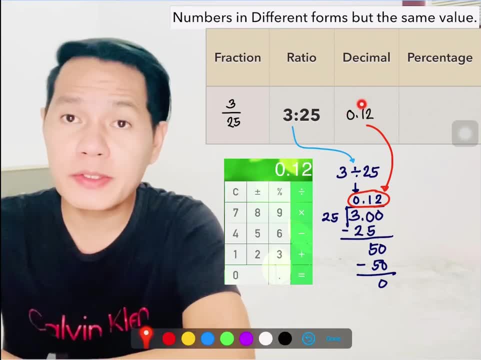 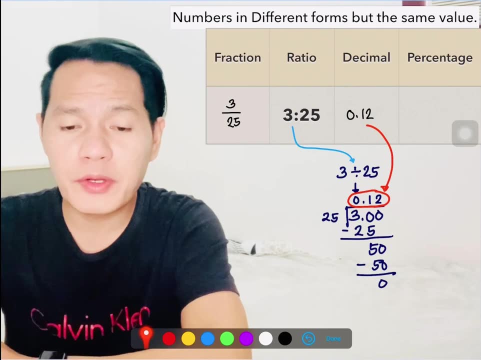 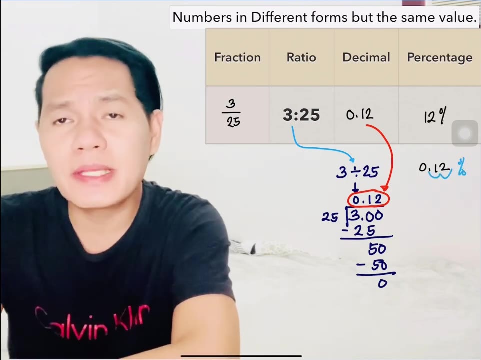 of the decimal, which is 12 hundredths or 0.12.. And then next into percentage. Okay, so we already have the decimal of 3 or 3 to 25.. So just simply times 100, or move it to the right 2 times and then put the. 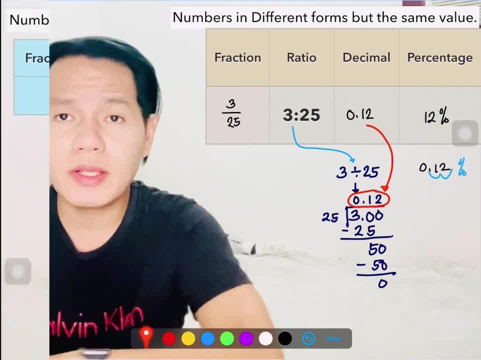 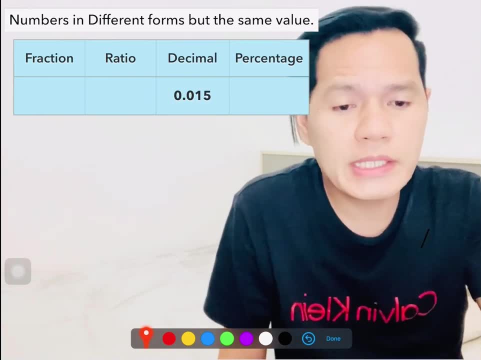 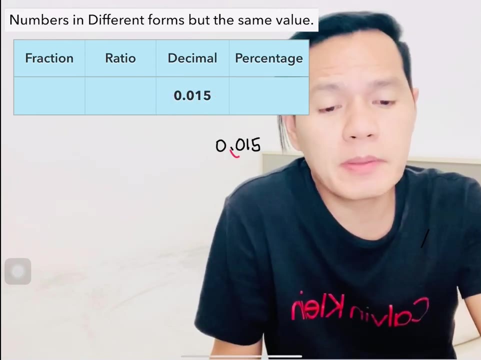 percent symbol. Okay, that's it. next one And the next example here is: given the decimal, the first thing to do to change this into percentage Just very simple: Multiply it by 100, or just simply move the decimal point to the right two times, and then don't forget to put the. 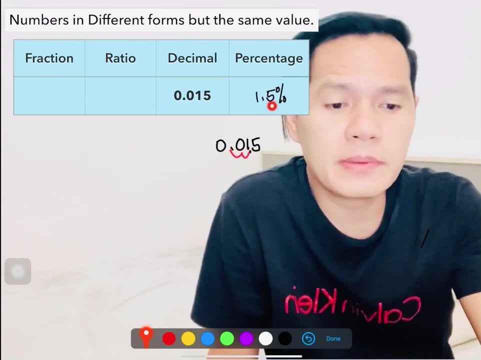 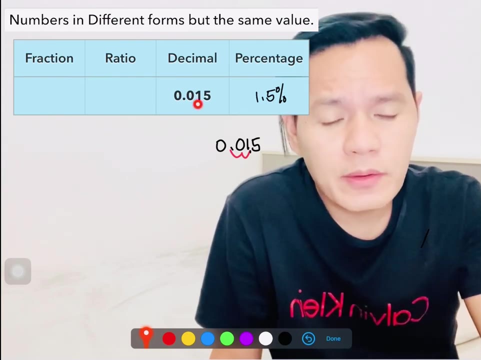 percentage sign or the present symbol. okay, and that's it. that's how you do it. and then next one is how to change this into ratio or into fraction. just go back to the decimal, which is: we read this one as 15,000, in other words, you, when you write. 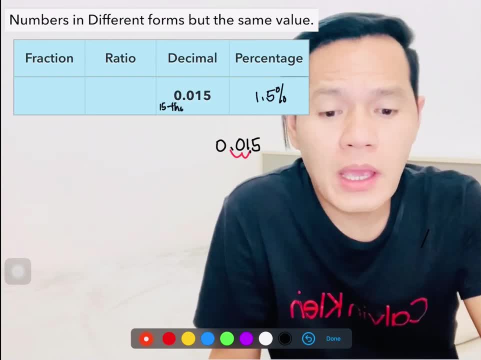 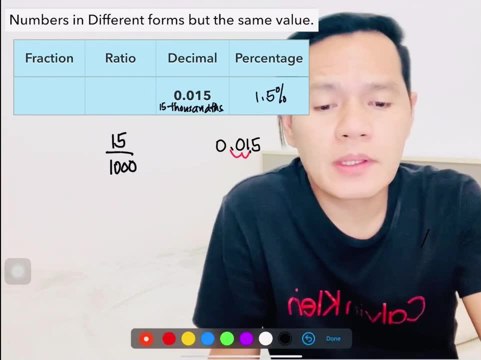 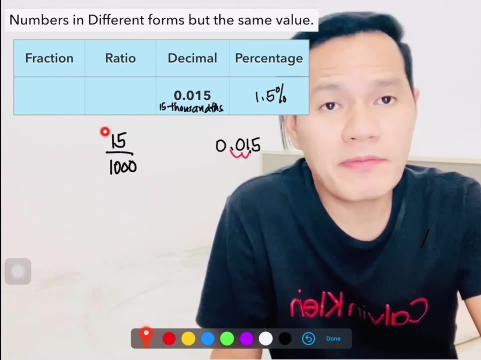 it in a fraction, it will just be 15 over 1000. so that's how you do that: 15 over 1000. and then, of course, since we are dealing here with fractions, do not forget to simplify your answer into lowest term. okay, so you have to reduce.